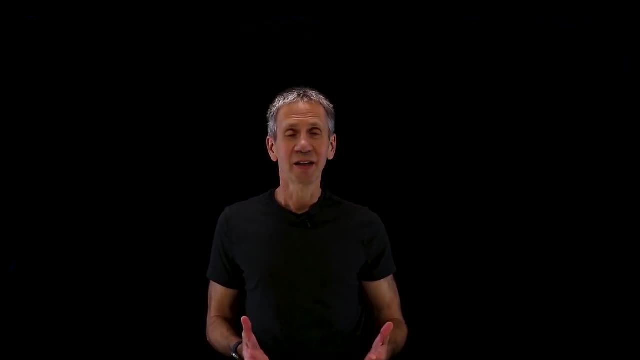 Your systems are up in smoke, or at least it seems like that. Nothing is working, The CPU is at 100% and you don't know why You can't get anything done. Well, what's happened is you've been DOSed. That's a denial of service attack. In a previous video I talked about 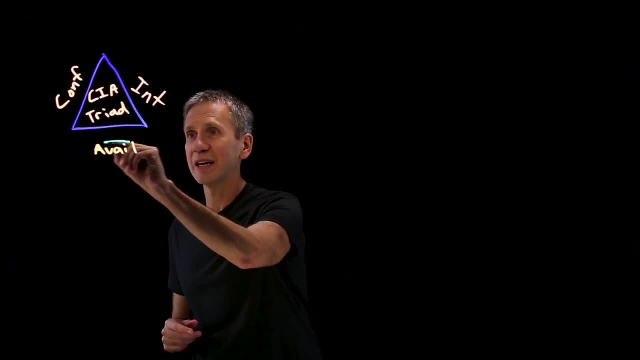 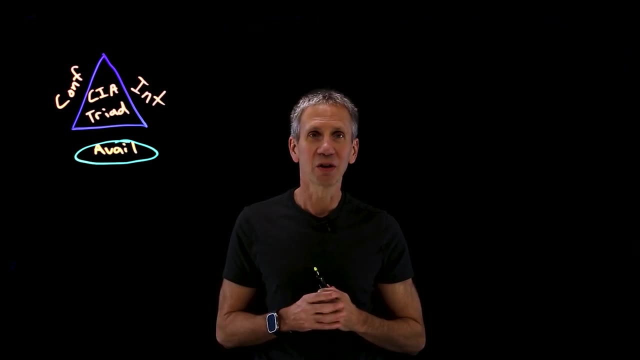 the CIA triad In particular. one of those aspects was this business of availability. A DOS attack, denial of service- is an attack on the availability of the system. Let's drill into that in a little bit more detail and find out what could be. Well, it turns out. 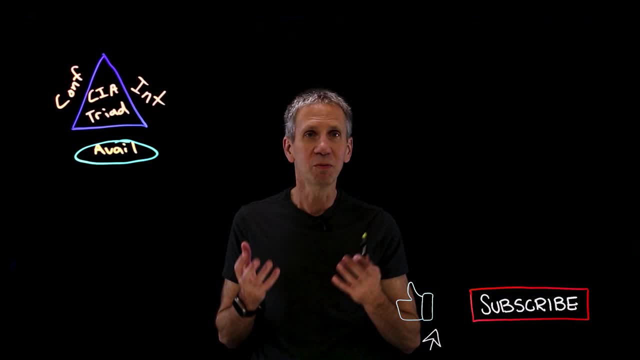 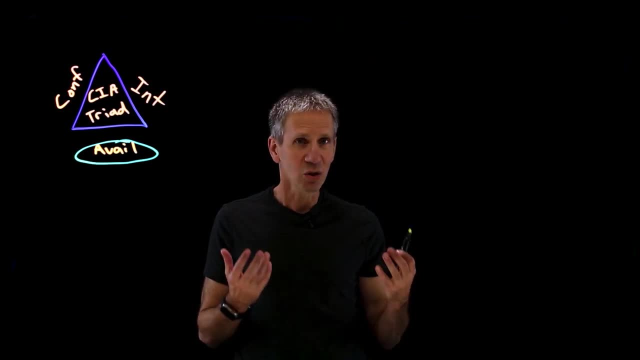 not all DOS attacks are the same. Most people tend to think about one particular type, which I will talk about toward the end, But in fact there are different classes of denial of service attacks. So the first one I'm going to talk about is sort of I'll refer. 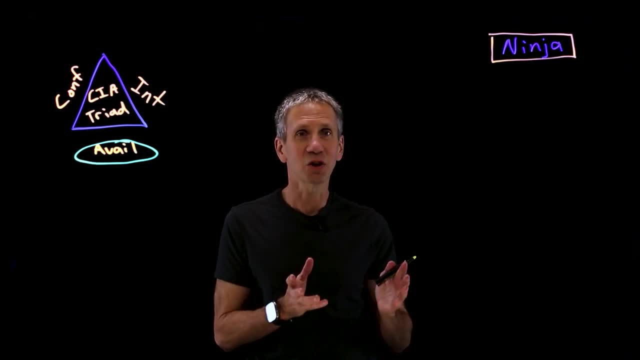 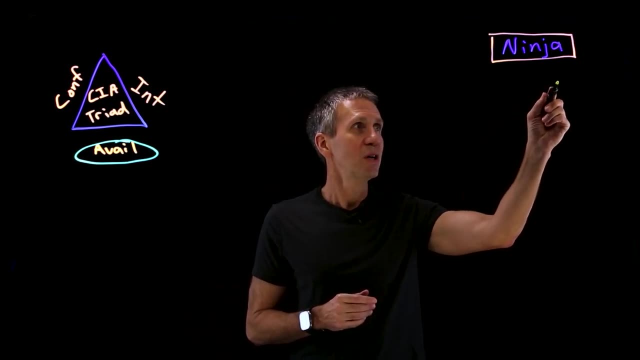 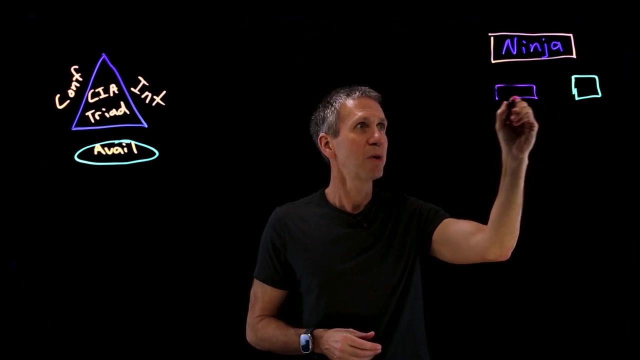 to it as a ninja attack. It's a surgical strike, It's a magic bullet, whatever analogy you'd like to use, But it's a very targeted strike And in this case what we do is we have a particular system here that's operational, and the bad guy comes along and sends a specially 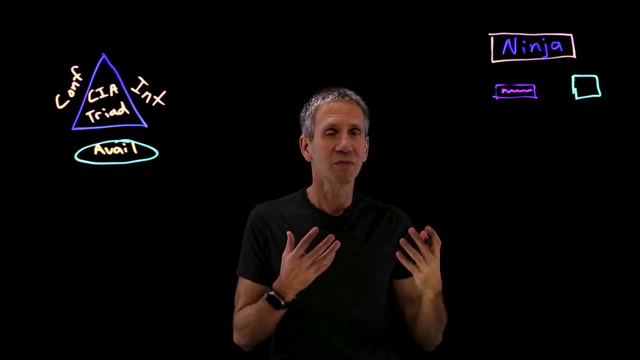 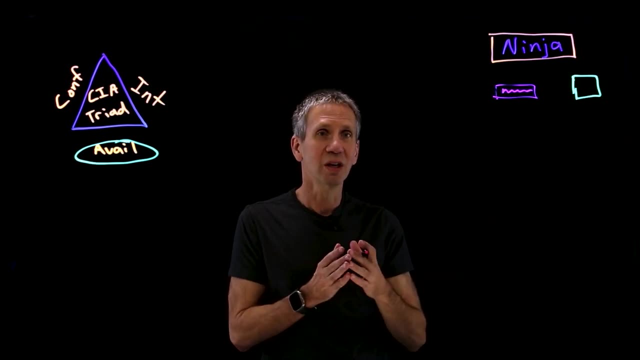 crafted message. So he's taken advantage of some rule that he's going to violate in the protocol, or he's using a buffer overflow, which is he's allocating. he's sending more information than was expected in the particular buffer where it was going to be received. 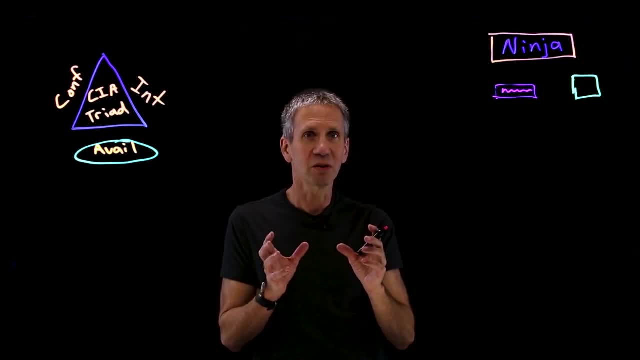 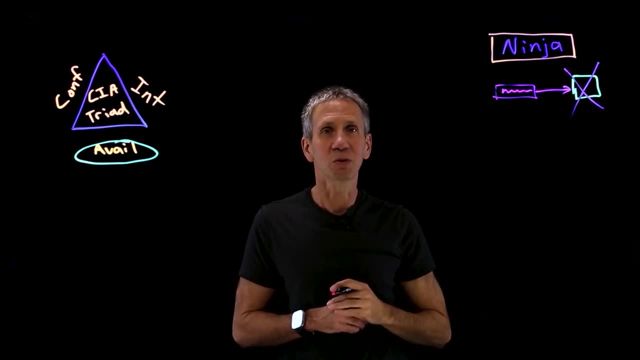 In some way. this packet has been specially configured and specially manufactured so that when it is sent to the target system, the target system goes up in smoke. It's one strike and the system is down. That's a type of denial of service that not a lot of people 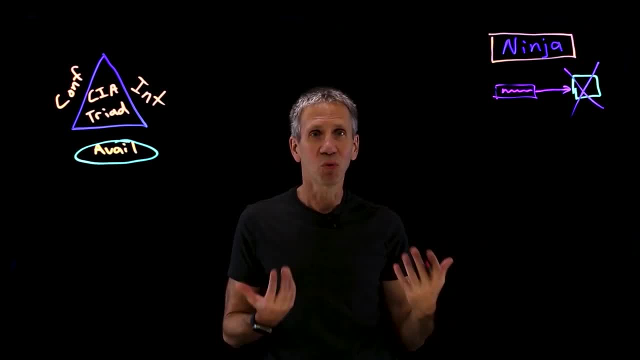 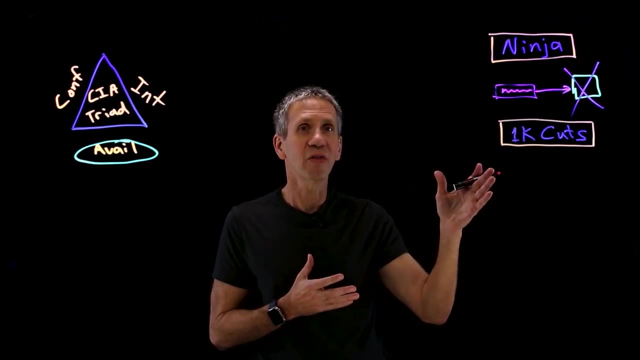 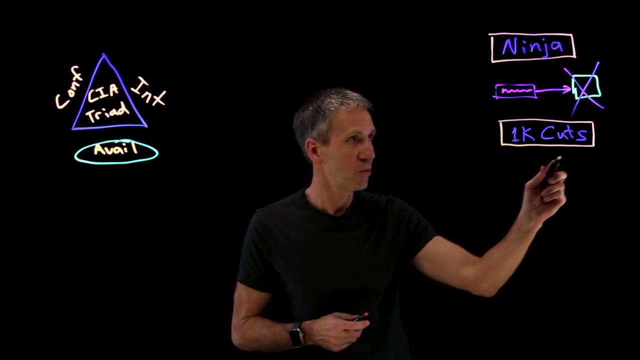 think about. They generally think about overwhelming with more volume, and we'll talk about that. That's the next type I'll refer to, which is what I'll call the death by a thousand cuts type of attack In these attacks- and there's a number of different types that can happen here. but 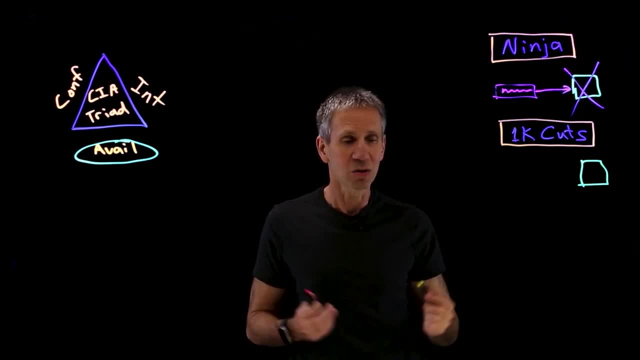 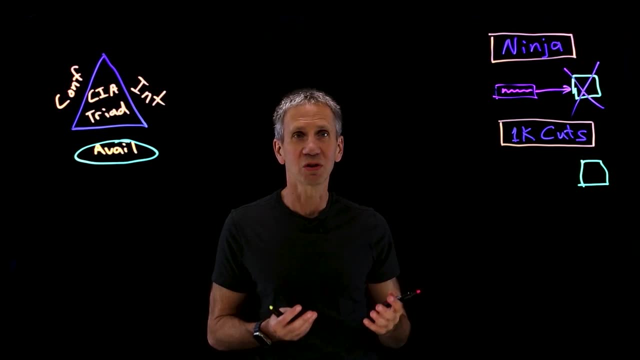 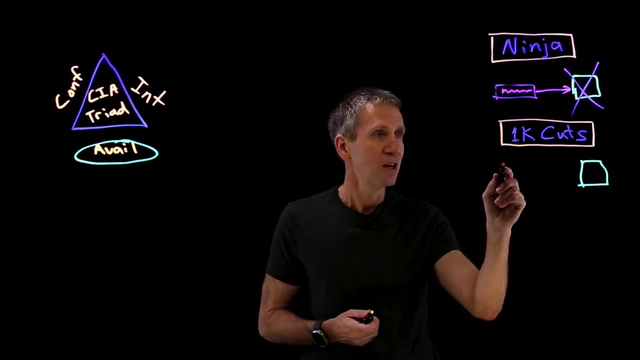 for instance. So here is our system. It's operational. I'll give you an example of an attack that dates back to about 1996, which was one of the early versions of this kind of attack, And it's called a SYNAC, or a SYN flood. What happens is a bad guy wants to take over this system. 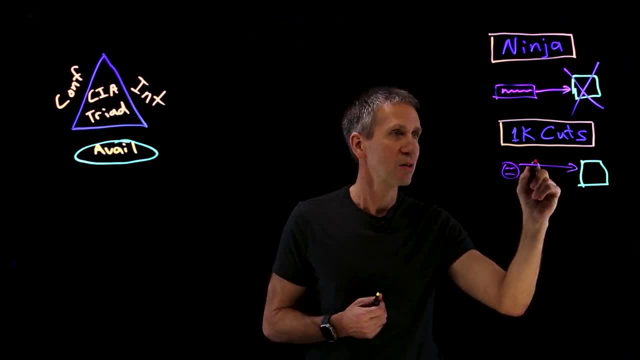 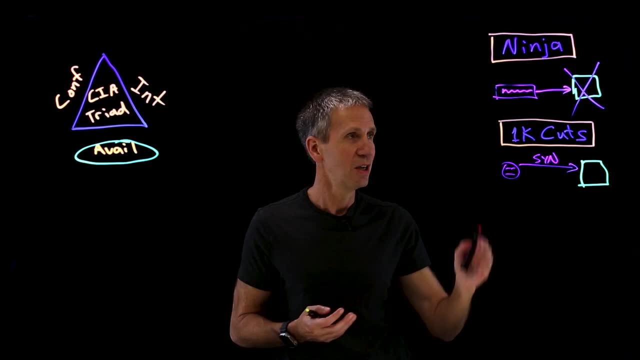 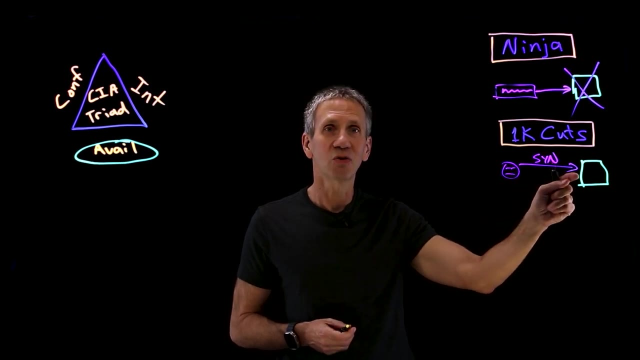 So what he's going to do is start by sending a packet. It's called a SYN In TCP terminology. this is starting what is a three-way handshake to begin a session. He sends the SYN message And what's supposed to happen in a normal case is he puts in his address so that the 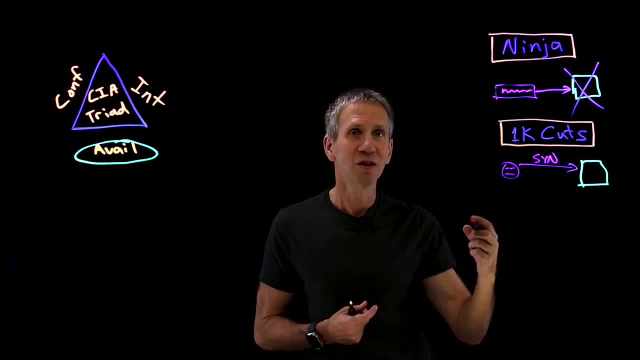 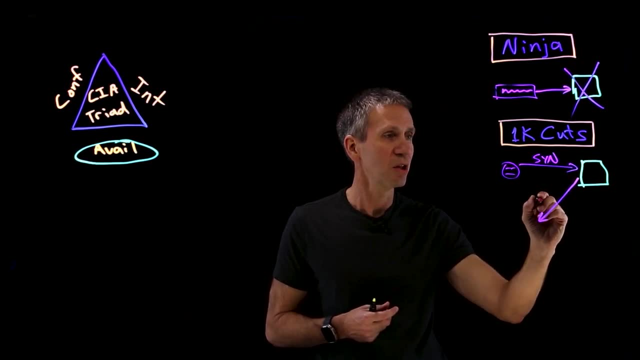 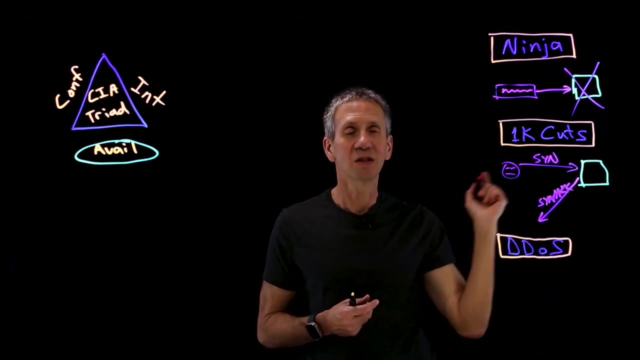 server responds with what's known as a SYNAC, a SYN acknowledgment. But in fact what he does, instead of having it come back to him, he sends the SYN acknowledgment to someplace else. He fakes out an address and says: don't send it to me, send it to someplace else. 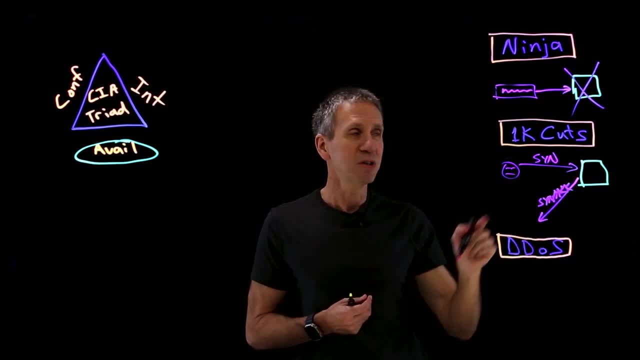 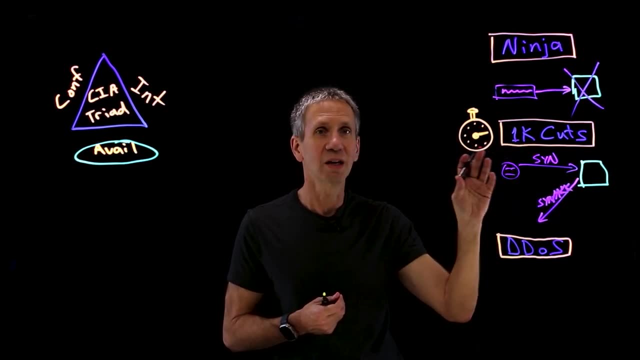 So he's lying about who he is Now. in the meantime, what happens is this system starts a timer And it allocates some resources for this new session that it's starting, And it waits now on an acknowledgment to come back from this place. Well, this place down here. 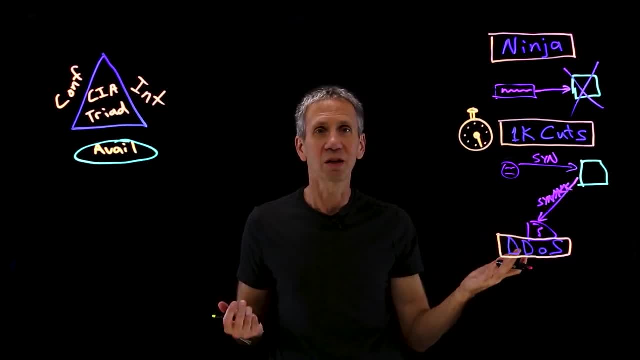 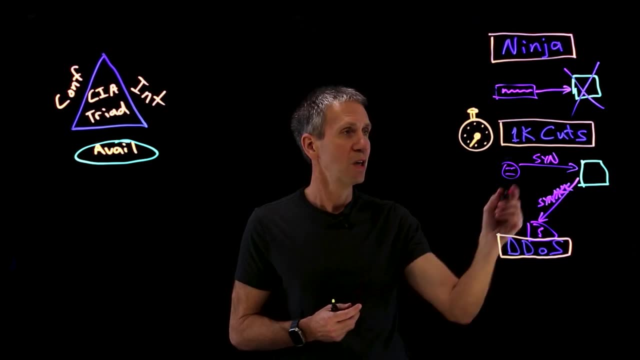 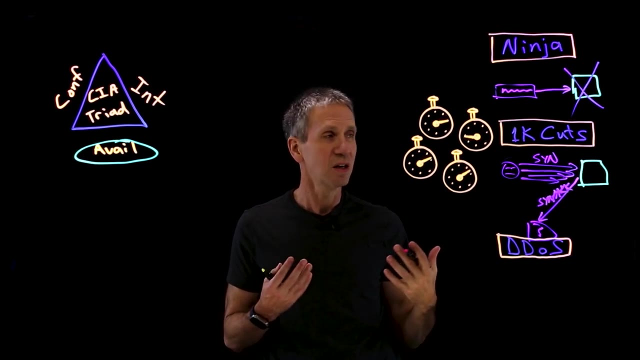 is unsuspecting. It doesn't know anything about this. It just got a random SYNAC message that it's going to discard, so it will never respond. In the meantime, this system is holding resources. The bad guy sends another SYN, And another SYN, And another SYN. It doesn't have to send a ton of these, but enough of. 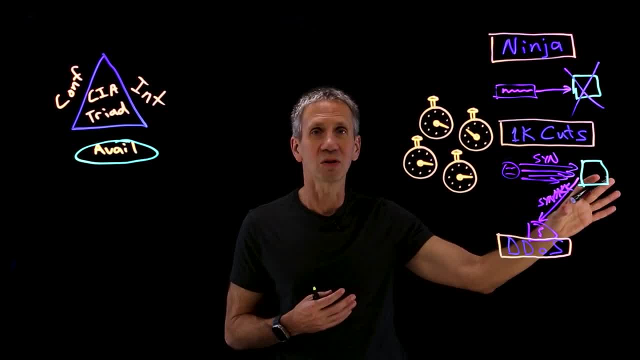 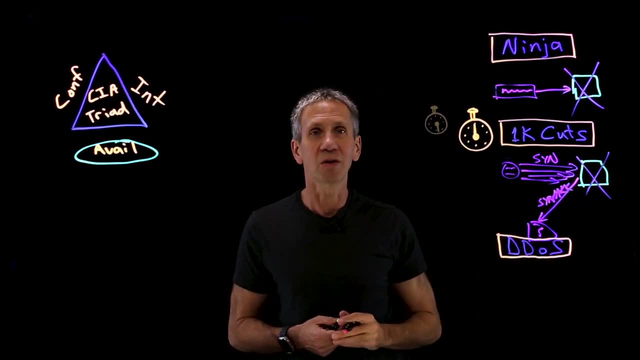 these where it's a death by a thousand cuts. No single one of these took the system down, But collectively, each one of them is reserving resources on this system until finally it's out Again. this was called a SYN flood attack And we have fixes for this now. People have adjusted, but the original TCP protocol did not take into account that someone might try to do something like this. There are other versions of this type of attack things. they do reflection, things that do amplification. You can look up if you're interested in something. 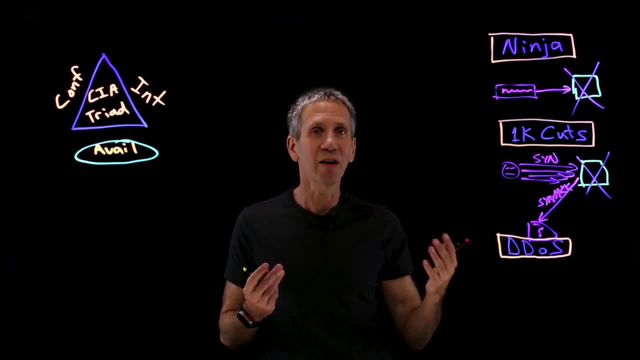 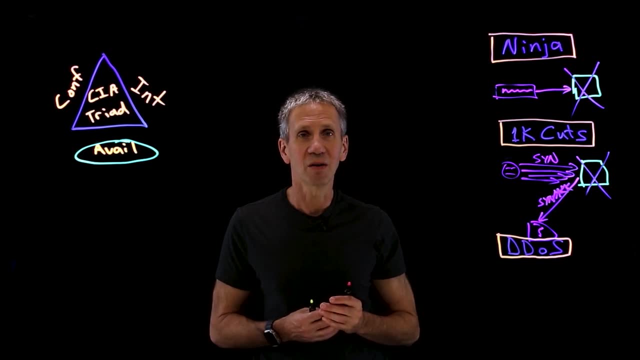 called a SMURF attack, which was of similar era. Again, we have ways to defend against these things now, but there are lessons to be learned as we look forward. So these are two different types of DOS attacks. How about the third major type of attack that? 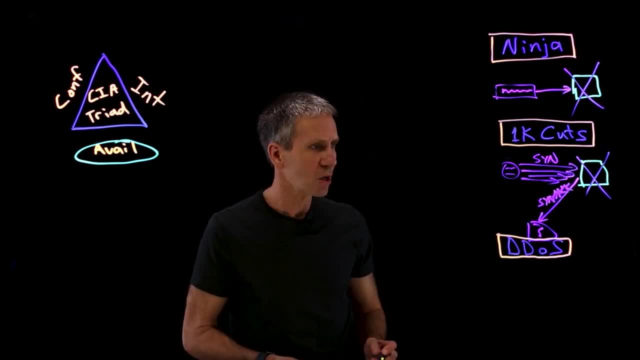 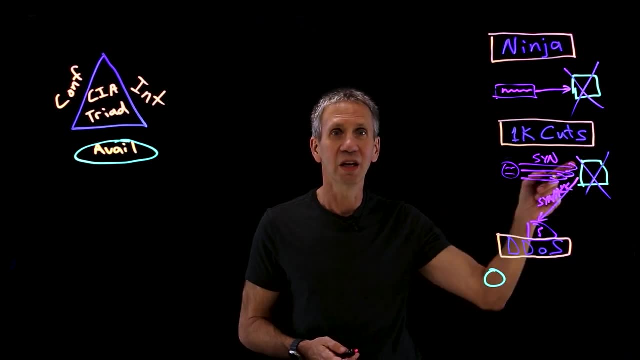 a lot of people are pretty familiar with, And with this one, what we have is we start with – this is basically a death by a thousand, where n is the number of users that are involved in the attack, And in this case it's going to be unsuspecting users. 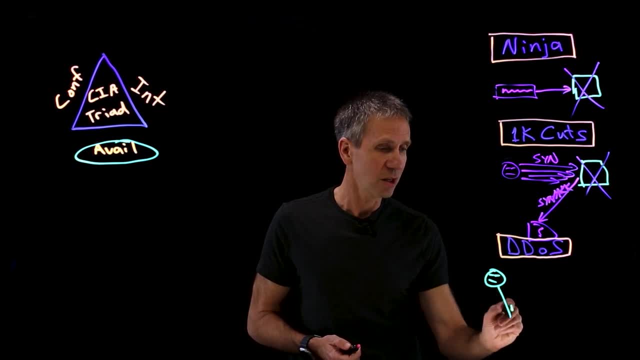 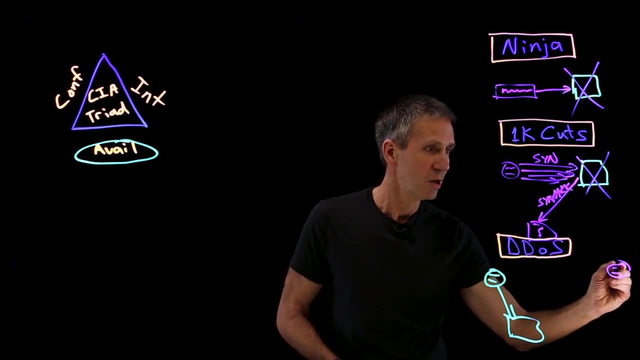 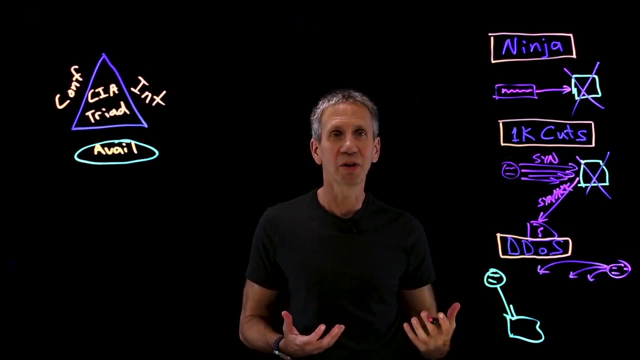 So we start off with one regular user who comes along, and they would access a system and everything's fine. In the meantime, a bad guy over here, though, is starting to take over systems. He has sent out some malware, or he's hacked into a bunch of systems, and 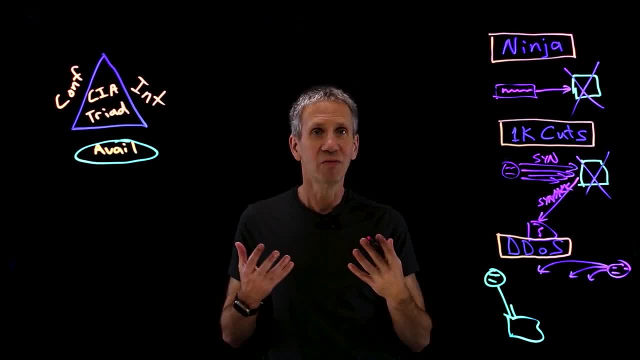 he's building what is now effectively an army of unsuspecting users that he's going to later use in his attack. We call this a botnet, or they were called zombies at one point, But these are basically systems that are sitting here that the user has no. awareness that they have latent code that could be exploited. Then, when the bad guy wants to start his attack, he sends a message out to all of the systems in his bot army And then they all start bombarding this system with traffic until it is way too much for anyone to deal with. 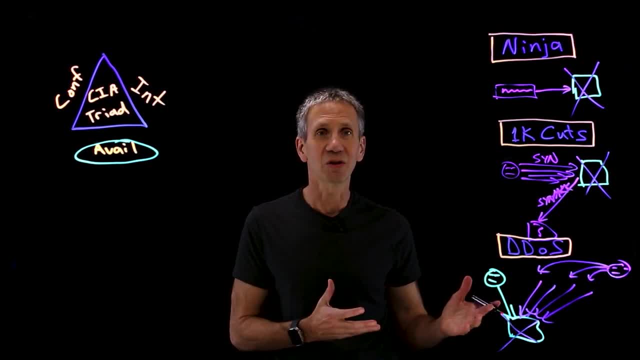 This is what's called a distributed denial of service attack, a DDoS attack. It's distributed in that, unlike these, the attack was coming from one place. In this case, this guy is just sending the command to start the attack. but 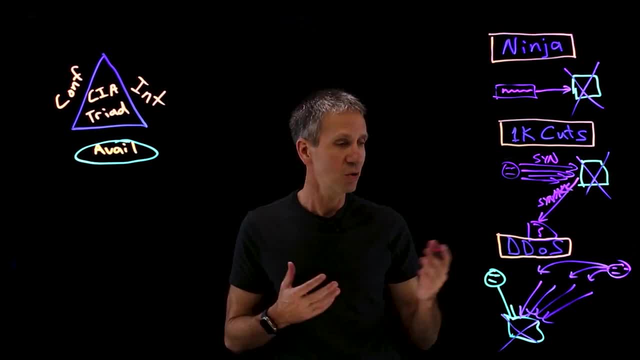 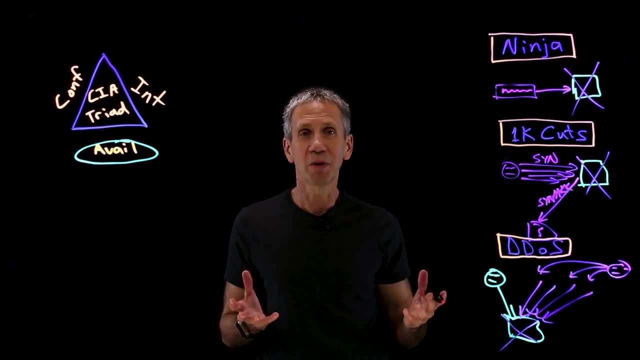 the attack is really emanating from a lot of different places, So that's why we call it a DDoS attack, And there are botnet armies that sit out there right now, today, that can be used by a bad guy. All he has to do is wake them up and send them on their task for a particular target. 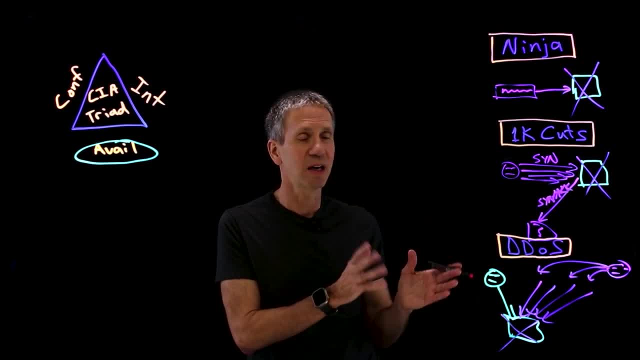 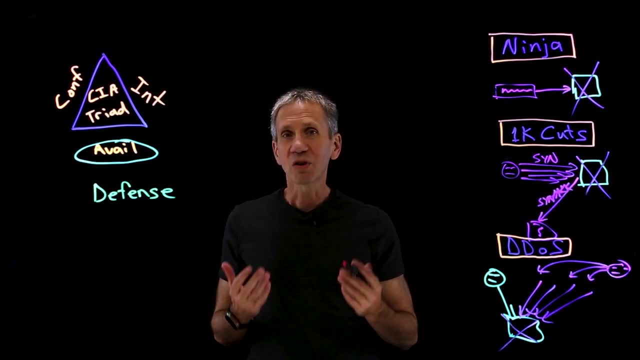 Okay, that's the scope of the problem, And there are many other types, but that gives you a general sense. What can you do about it? Well, it turns out there's a number of things, So let's look at some defenses here. 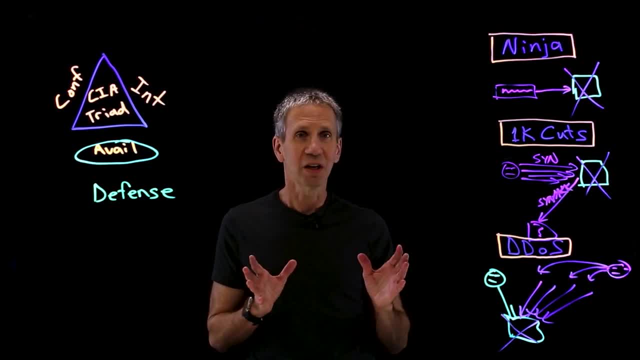 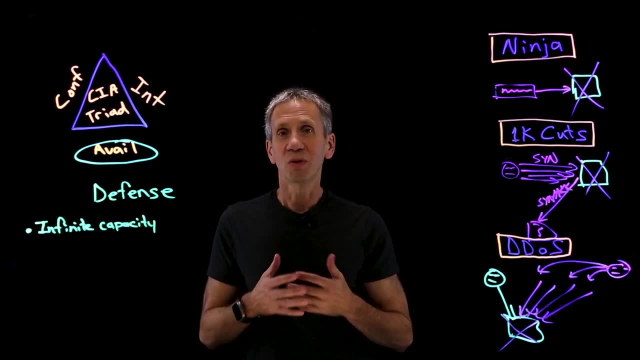 First of all, the number one defense for any sort of denial of service attack- and I'm going to say this facetiously- is infinite capacity. Unfortunately, nobody can afford that. So if you had infinitely capable systems, then you could throw as much as you wanted to at them, and 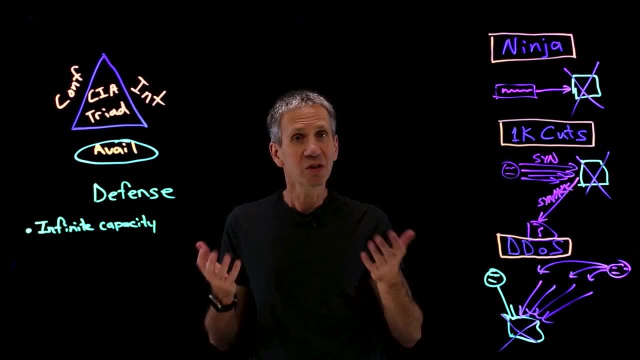 they would be able to withstand the attack, but that's too expensive. What's the next best thing? Redundancy. If you have only one system, then one system is a single point of failure. If you have multiple systems, for instance, in most cases 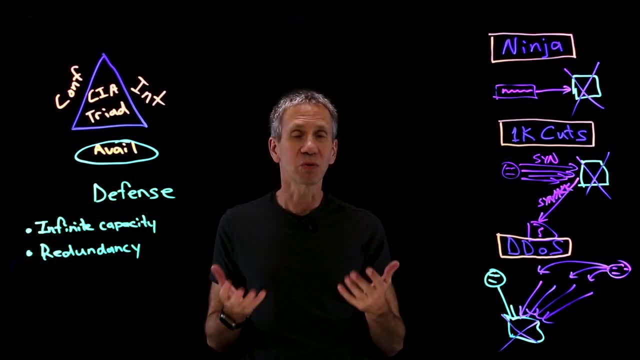 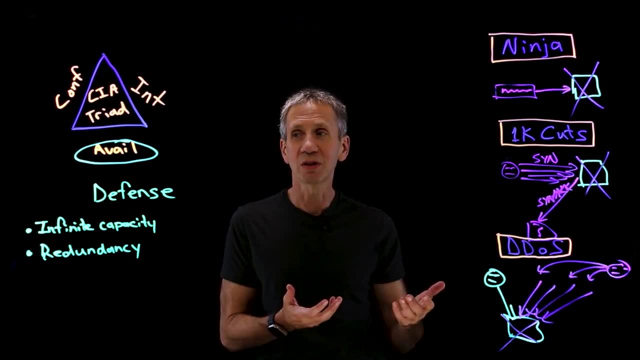 we use what's referred to as the rule of three, where you want to have at least three of everything. So if one goes down, you're not at 50% capacity, You still have what is a a usable, a usable system. 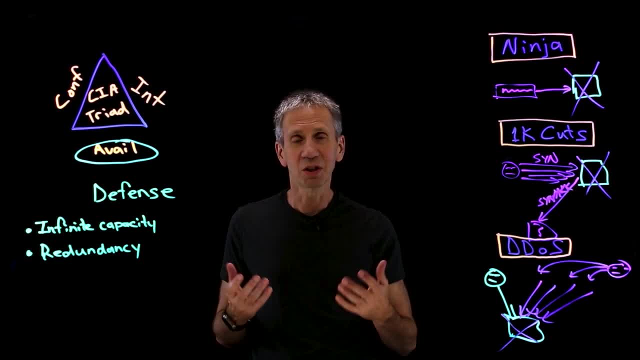 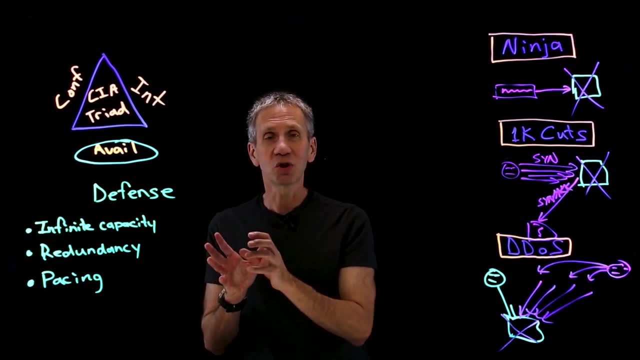 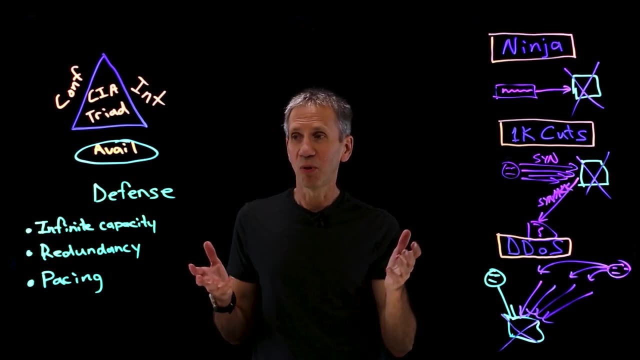 So redundancy is another important part to have here. Adds to expense, but it's necessary. Pacing, that is, looking at the traffic as it's coming in and limiting how much we will accept over a specific interval of time or traffic going out, which also comes to the point of filtering. 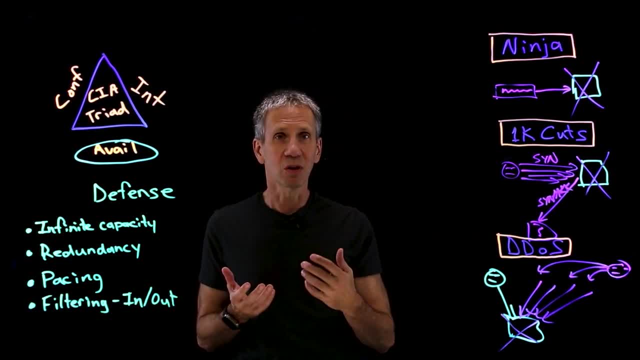 Now, in some cases we want to filter traffic coming in from certain locations, from certain IP addresses. We want to be able to turn these filters on when we know we're under attack, and we- and it's very difficult to do that in a DDoS attack. 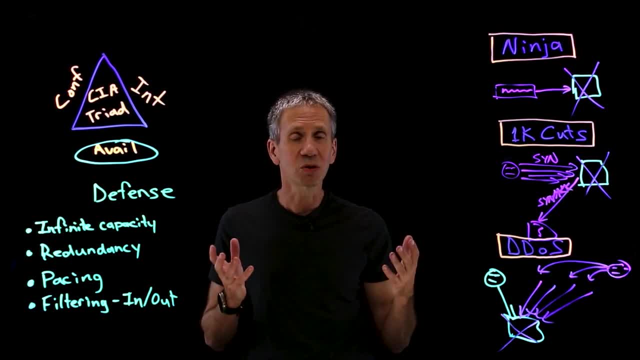 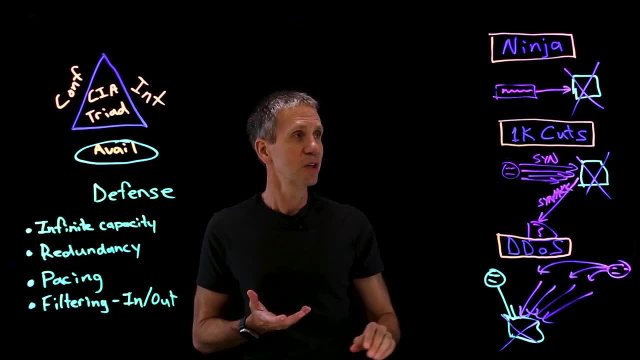 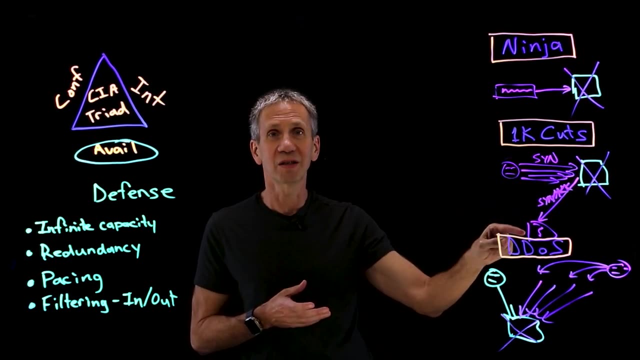 because the attack seems to be coming from everywhere. We should also, as responsible citizens, be looking at doing egress filtering, or filtering the data that's going out of our systems. For instance, if the ISP for this guy was looking and seeing that he was sending lots of SINs that were referring to an address that's not him. 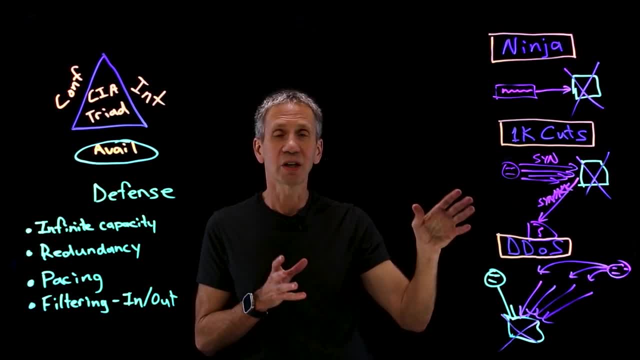 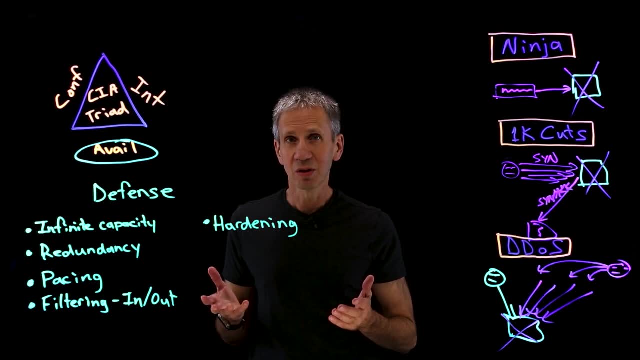 they could have blocked that at the source. So the right kind of filtering as the egress helps everyone. if we do that kind of thing, Okay, Okay, Okay, Okay, Okay, Okay, Okay. Other things you could do would be harden systems. 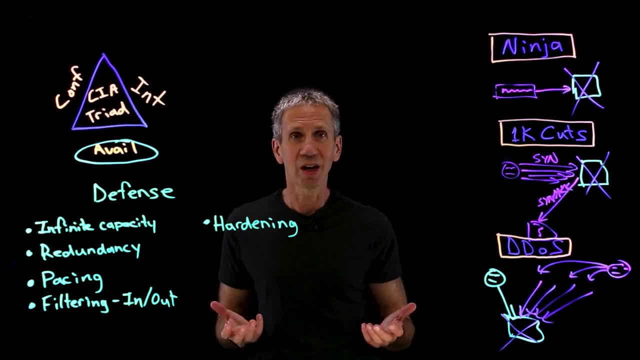 That means remove unnecessary services, remove IDs that are not needed, remove capabilities that are not going to be used. Every one of those is something that a bad guy could ultimately exploit later, So we don't want to have anything that's not absolutely necessary on the system. 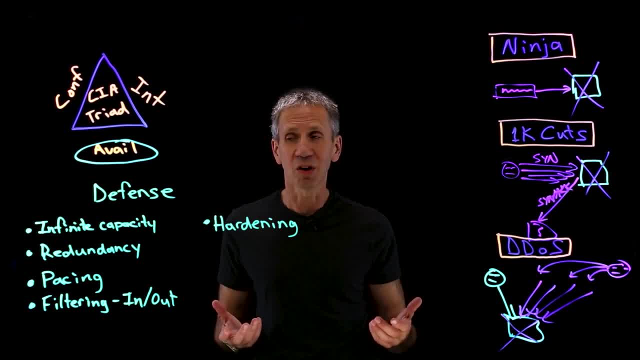 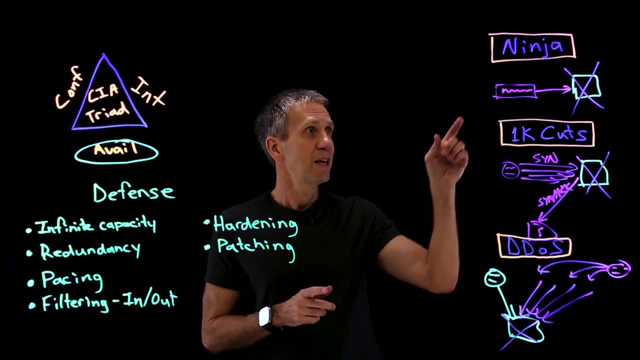 We also want to change default passwords and user IDs if at all possible. Patching is another Making sure that all the systems have the latest software on them. It's software fixes that took care of a lot of these earlier DOS attack scenarios. 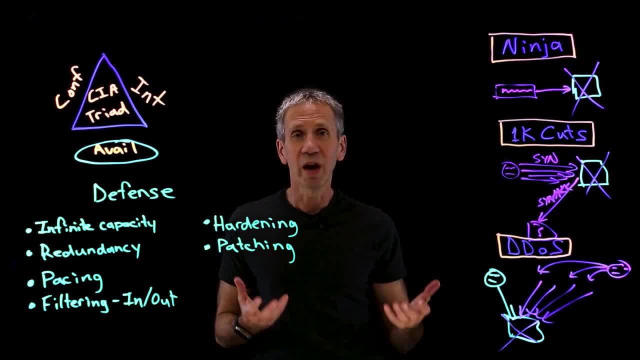 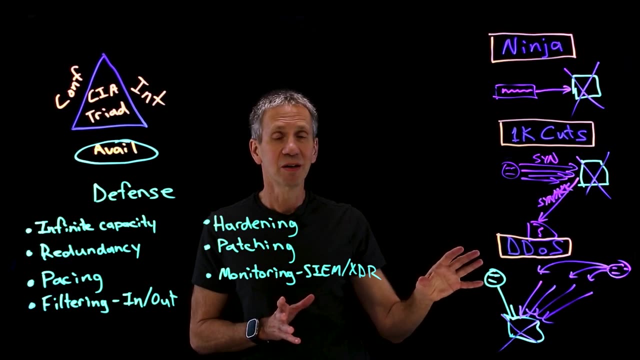 So the vendors will continue to find ways to fix their products, and we need to keep our capabilities up to the level of where those fixes are: Monitoring, being able to look over the whole system and understand when this is happening and when it's not. 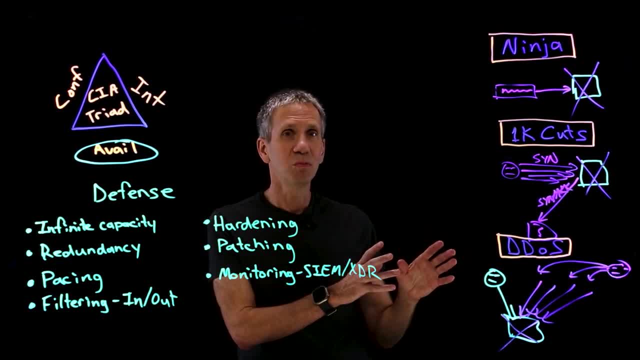 Understand. is our system really under a load because we're being ultra successful right now- Maybe we just put some new product on sale and everybody is there- or is it because a bad guy has decided to try to take the system down? We need to be able to understand the difference between the two.